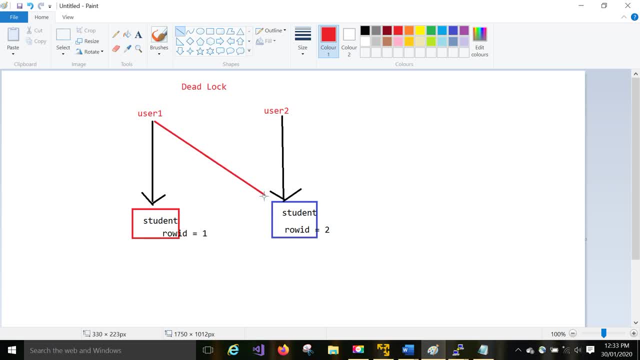 This guy will try to Update Same row. Same row is trying to update that. This guy, This user 2. Is trying to access This row 1., Same row. Ok, What is happening here? User 1 is trying to access row id 2.. 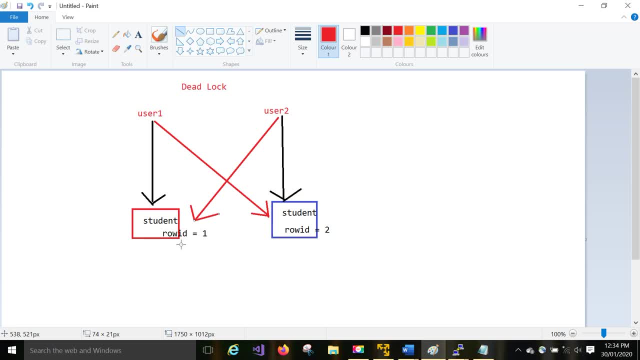 User 2 is trying to access row id 1.. Before that, only he is working on row id 1.. And before that, this guy is working on row id 2.. This is the thing happened In this case. Then automatically this guy is trying to access this one. 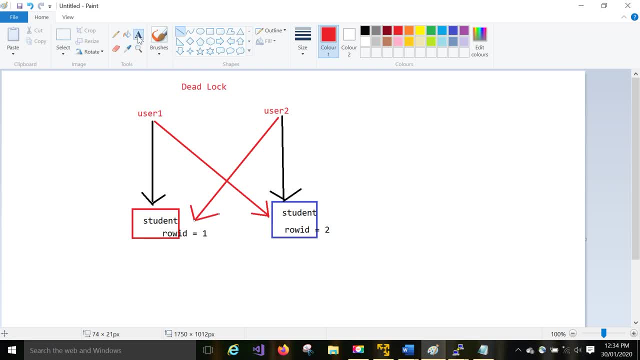 This guy is trying to access this one, Then you will face a deadlock here, Deadlock here. That is the thing. This is not like a DBA related, This is like a development side. But you have to identify, Ok, Whether 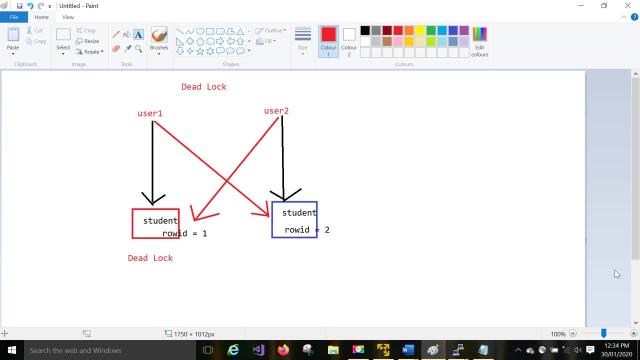 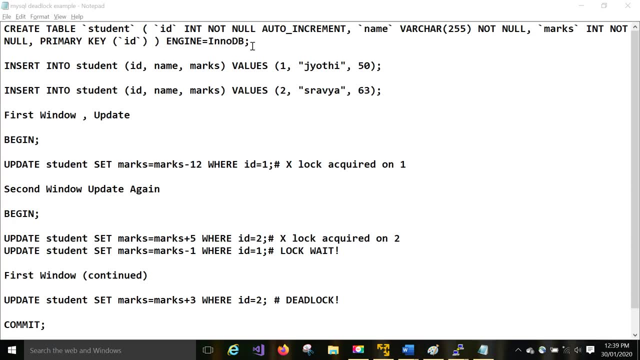 Deadlock is happened or not. You have to identify that. Fine, I will show you the example. Here you can see the example. I am creating a table And inserting two records. Ok, See, here I am in User 1.. 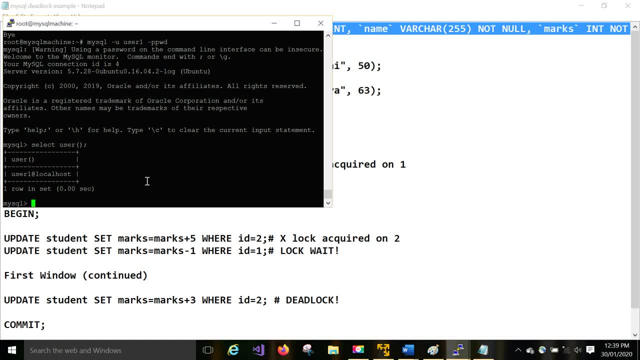 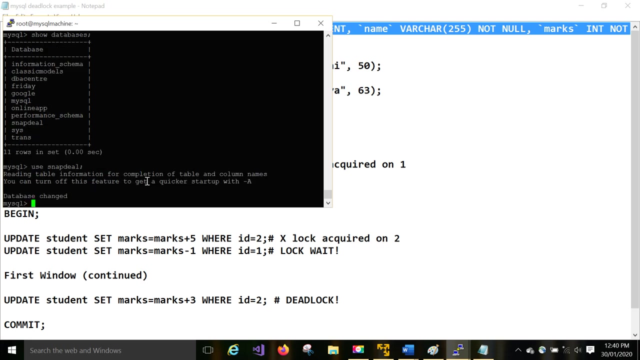 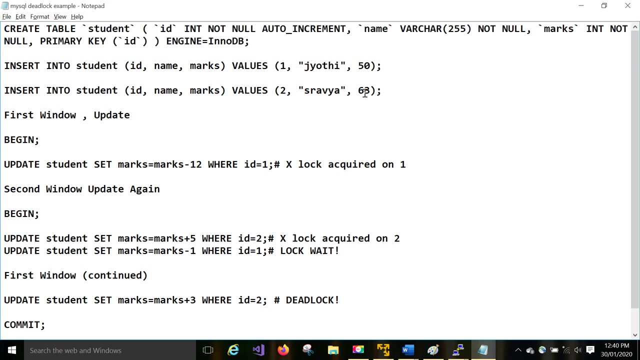 Which database. you can use. Any database you can use. Show database, Show databases. You can use snap deal: Ok In this. you can use this one Creating. Insert two records, Ok, Id 1. Id 2.. Insert two records. 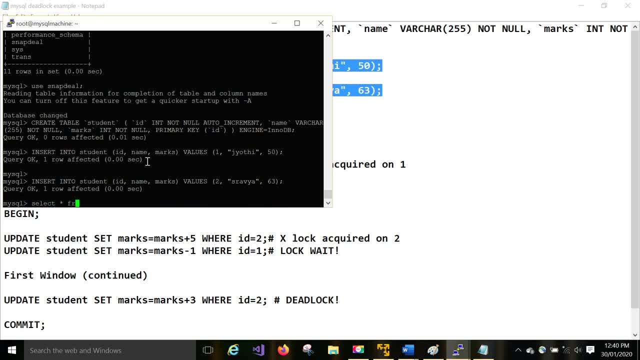 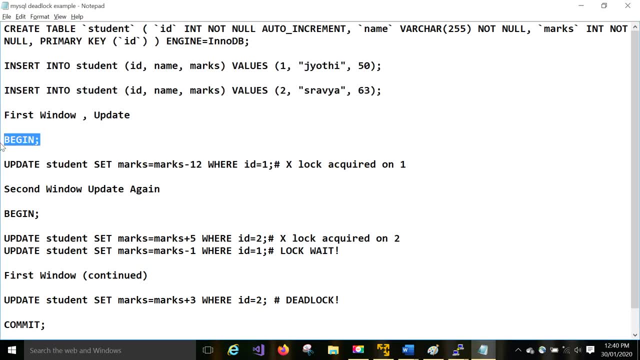 Done. Then select and verify that Normal. These two records are there. Now Go to the begin statement To do any transactions. If you want to do Begin transaction. Updating Id 1.. You are updating Id 1.. 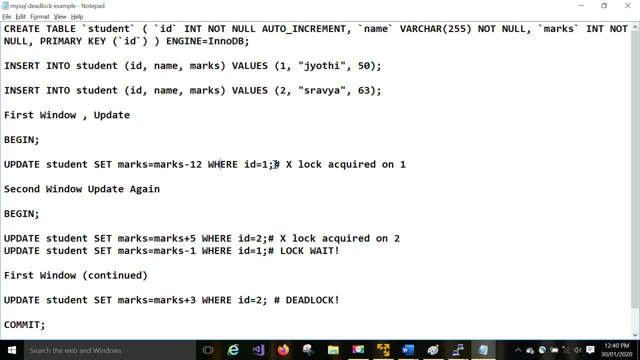 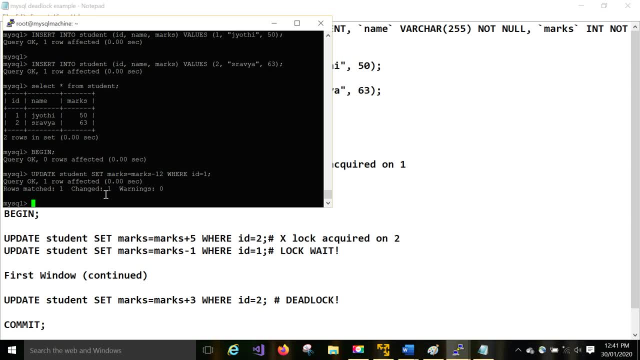 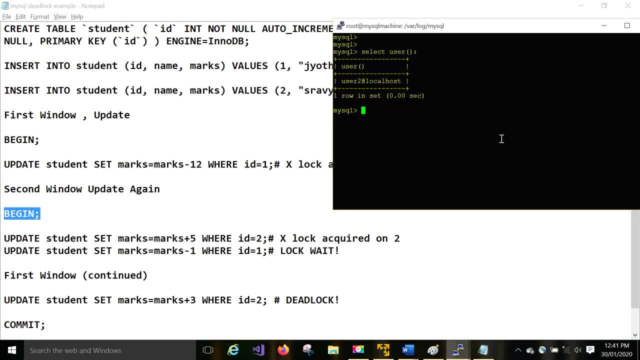 Marks Minus 12.. Ok, Updated. Obviously Open second window. See The first one. Second is doing Is activity. I told right Second is doing On second record Is not. No See, Oh. 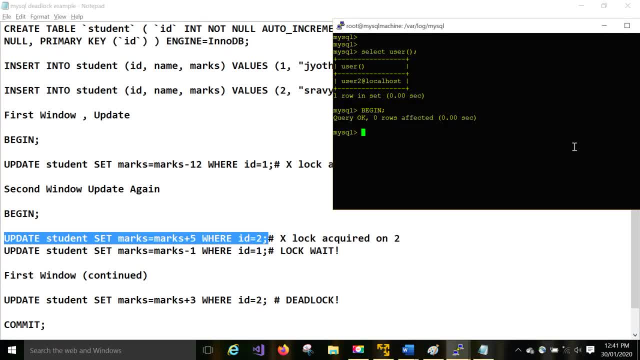 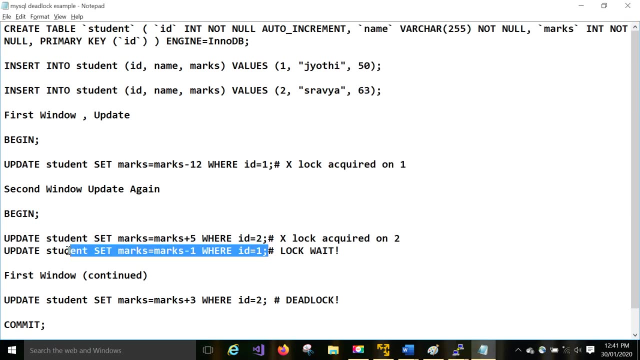 Sorry, You have to select Snap deal Database. Wait, Second record. He did Then again. You have to select Snap deal Database. Wait, Second record. He did, Then again. He is trying to access first one. 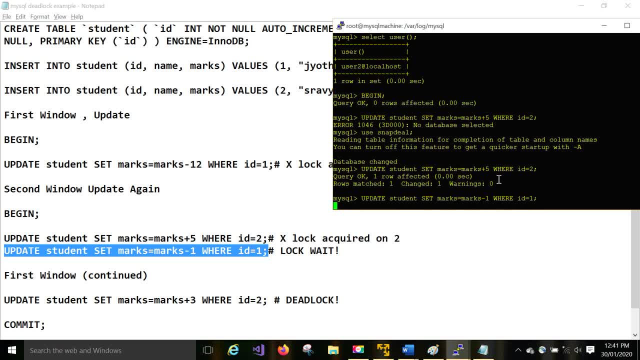 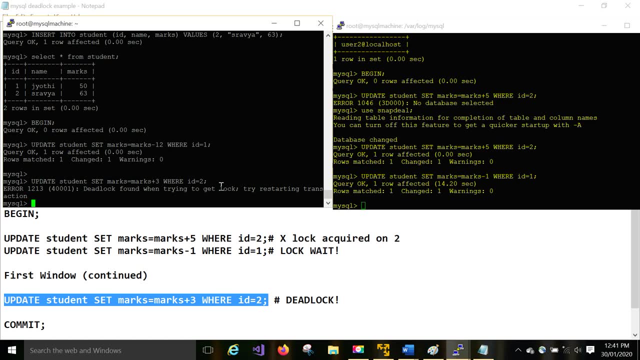 See this. It is Why, Because of already that guy is working on that, Then first window fellow Is trying to access On second one. See, Deadlock has been identified Like this. You can try example. Fine, I will give you the script in. 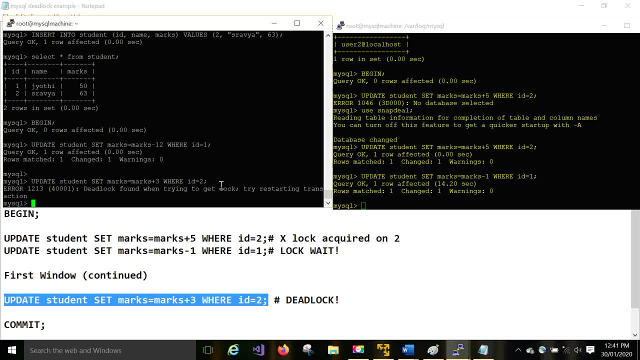 Below the comments, You can try on the exact. Then Fine, Your Boss is asking How to identify The deadlock Because developer to developer DBA cannot able to see that Right. Then how to do, I will show you. 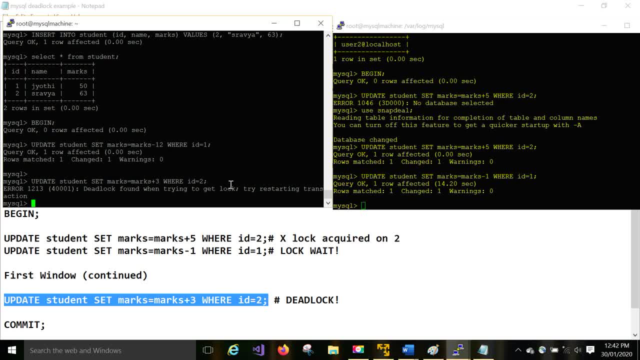 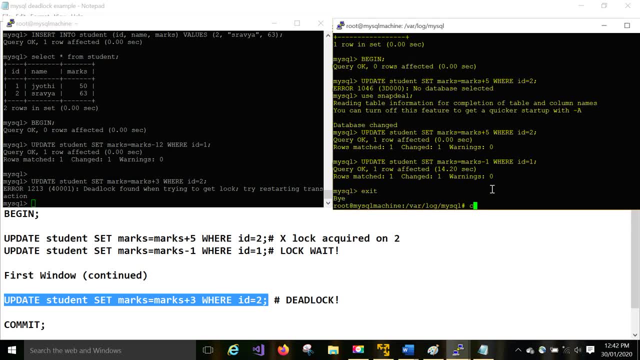 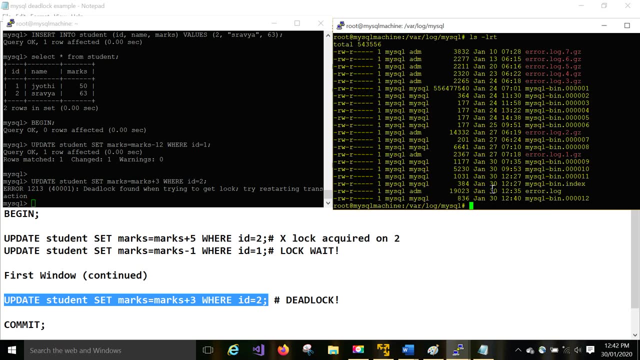 Let it be: First verify In your. It has to record In your Error log. So You have to First Verify In your. It has to record In your Error log. Error log. Go and see this. 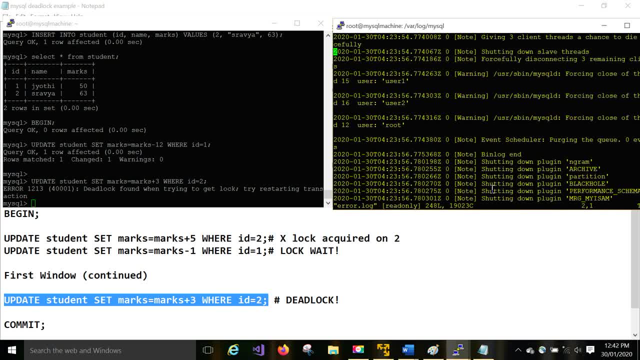 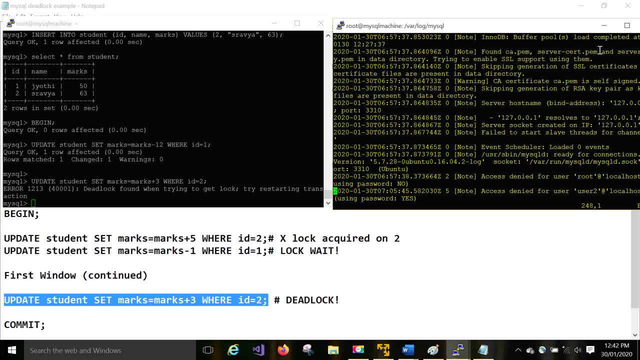 Ok, Shift to G Access denied something. It is there, But it Deadlock is not Showing here. It is not recorded Then How you should Do that If you want to record Whether Deadlock is. 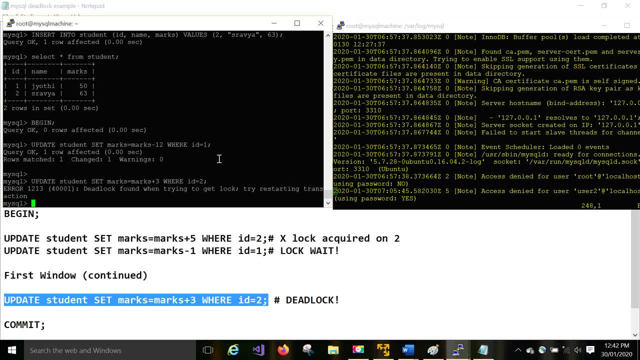 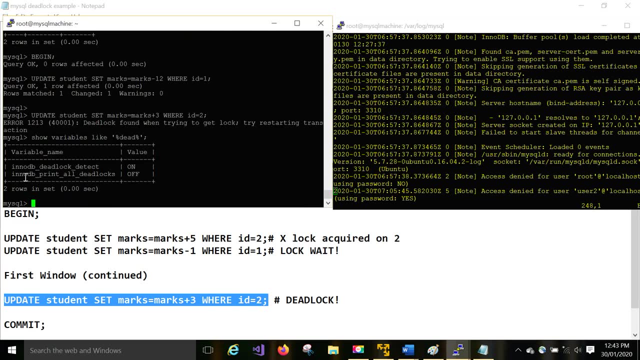 Happened Or Not. Show Variables Like Just You Can Give Like This: Ok, This Is Of InnoDB Print All Underscore Deadlocks: Ok, This.